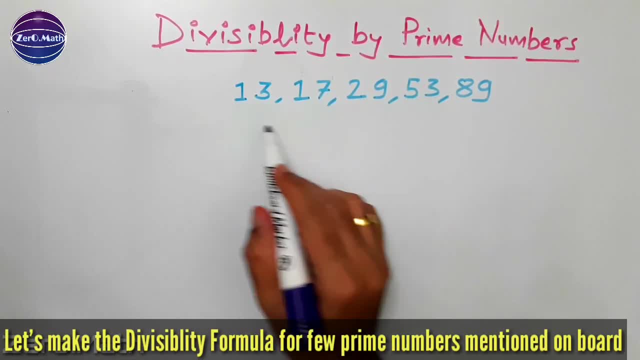 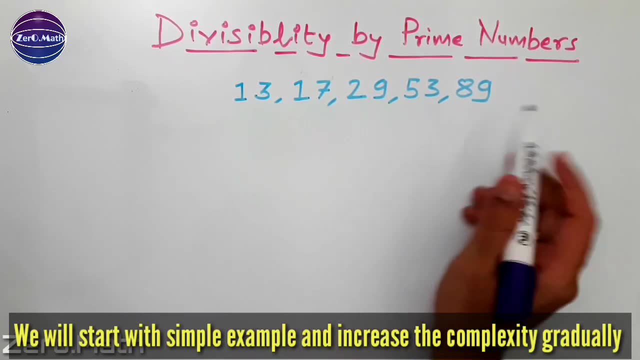 So, friends, let's make the formula, To make the formula of divisibility by these prime numbers. I am going to cover all these examples. However, I will start with the simple example and I will increase the complexity in each step. I would recommend you to watch this video in full so that you will not miss anything. 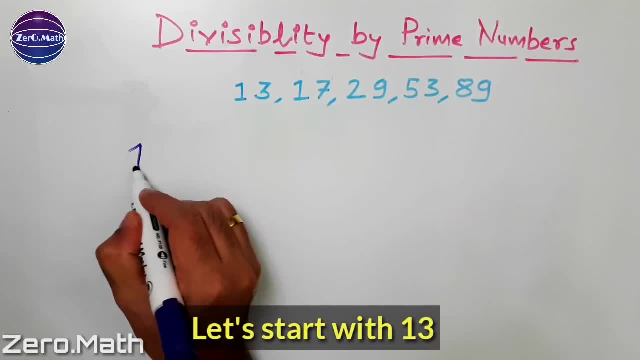 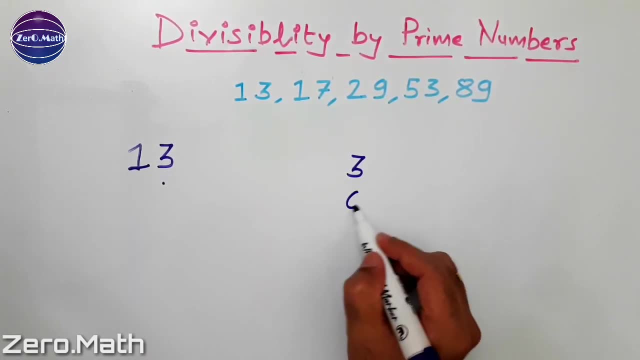 So let's make the divisibility formula for number 13.. So what I am going to do, I am going to take the unit digit number, that is, 3, and I will write the table of 3.. 3,, 6,, 9,, 12,, 15 and so on. 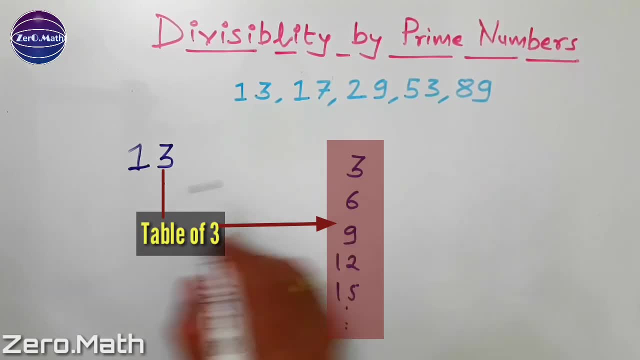 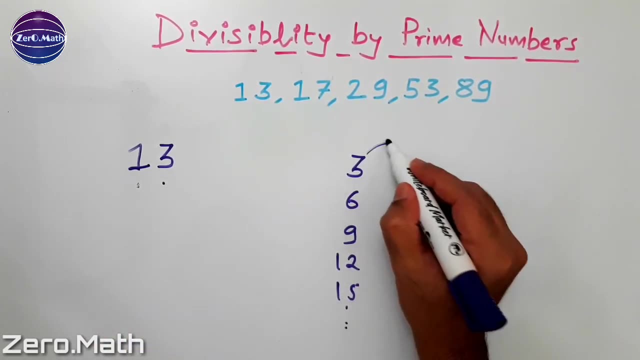 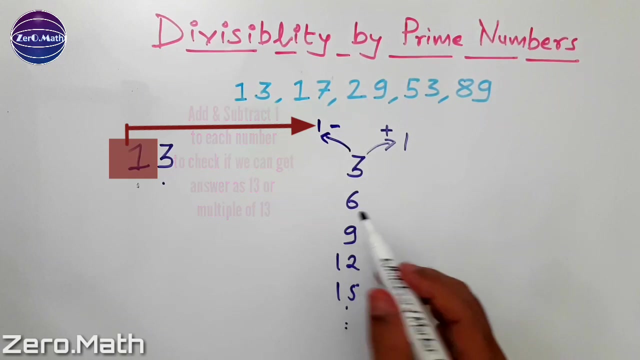 This is just. This is just for the sake of explanation. Then I will take the number which is at the 10th place, that is, 1.. So what I am going to do, I will add this 1 to each of the number and I am going to subtract this 1 from each of the number. 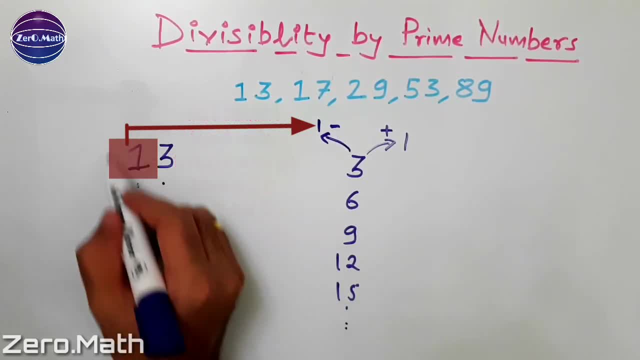 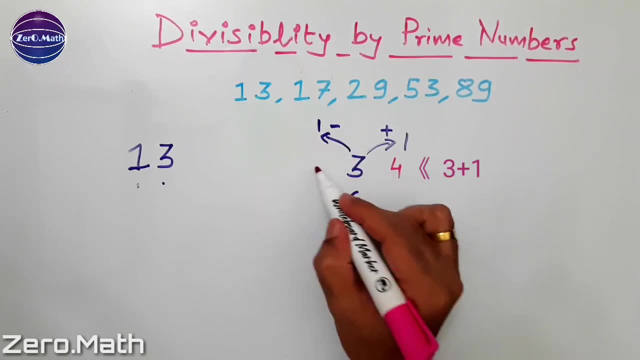 I am going to do this process till I get 13 as my answer, or multiple of 13 as my answer. So basically, 3 plus 1 is 4, 3 minus 1 is 2.. So this is not equal to 13.. 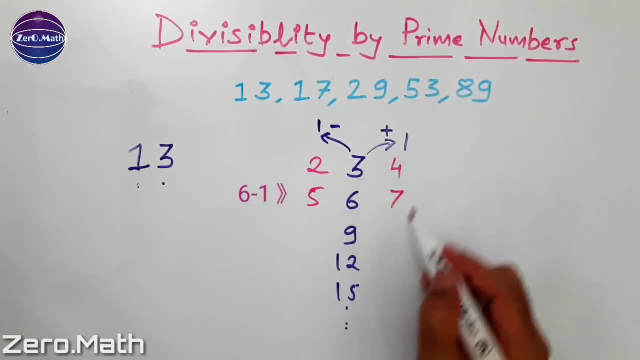 6 plus 1 is 7,. 6 minus 1 is 5,, not equal to 13.. 9 plus 1 is 10,. 9 minus 1 is 8,, not equal to 13.. 12 plus 1 is 13.. 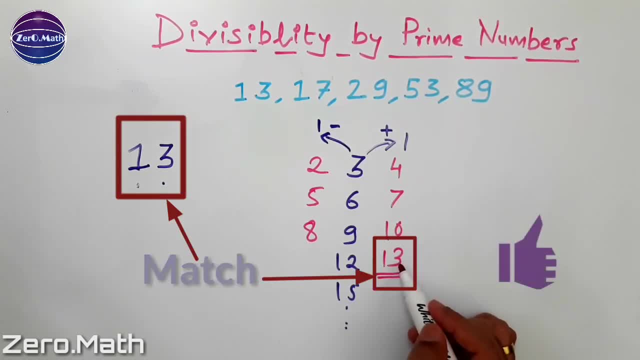 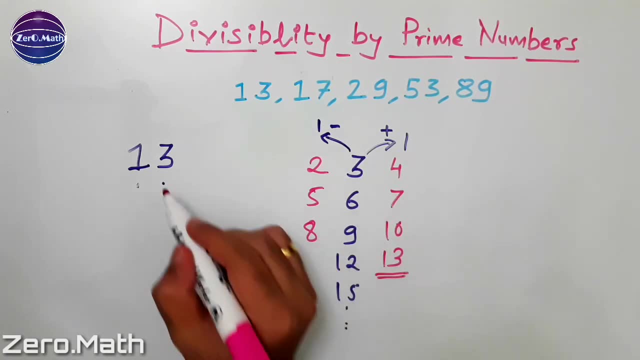 Yes. So here we go. I got result as 13.. So basically this is going to be my divisibility rule. So divisibility rule of 13 is 3 into 4 is 12.. So what I am going to do? I will multiply this unit digit number by 4.. 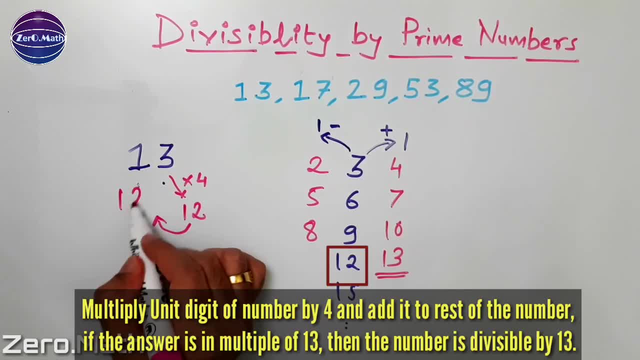 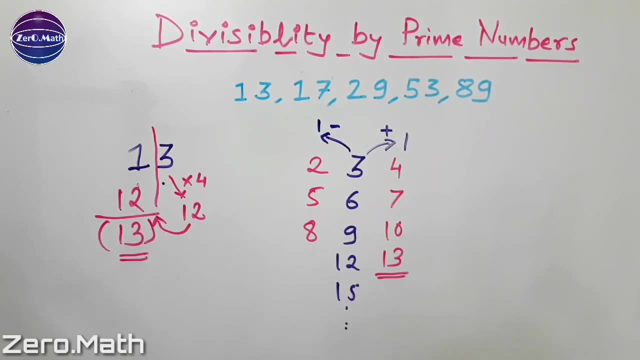 Whatever I will get, I will add this to Rest of the number and, after adding this, what I am getting. if this is completely divisible by 13,, then, yes, my number is completely divisible by 13.. That's the divisibility rule. 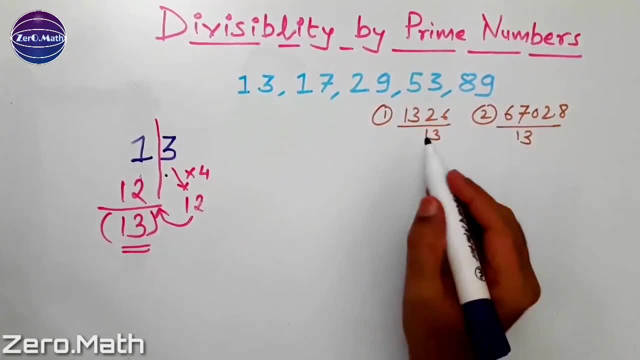 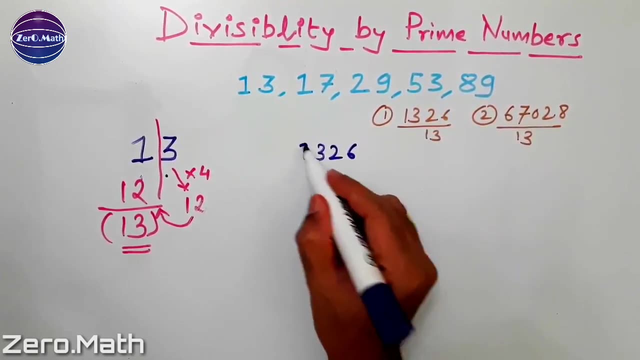 So let's test this. Let's test the divisibility rule of 13. Let's see whether number 1,, 3,, 2, 6 is completely divisible by 13. So let's apply the rule. Multiply this 6 by. 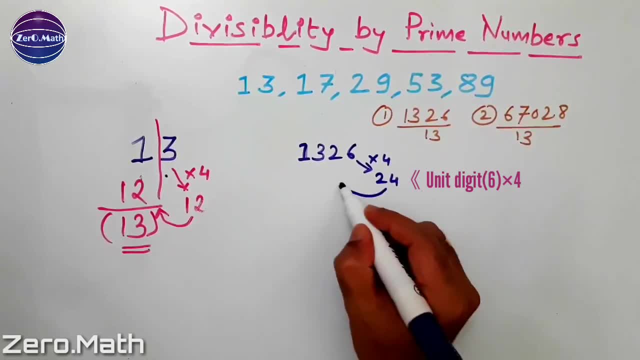 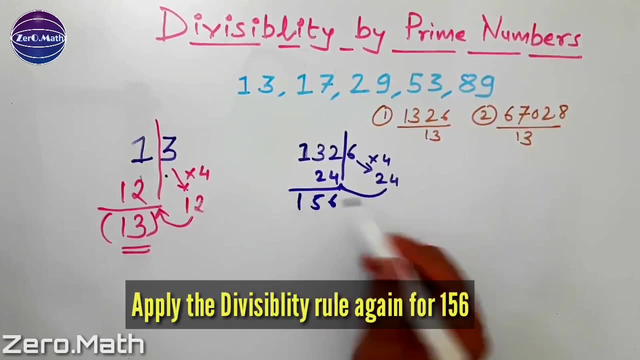 4,, which is 24.. And take this 24 over here. Add this to the rest of the number, So 2 plus 4 is 6.. 3 plus 2 is 5, 156.. Since I cannot make out whether 156 is still divisible by 13,, I will apply the rule once again. 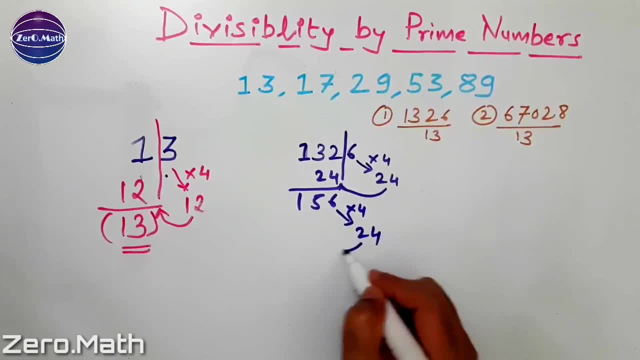 So again, I will multiply 6 into 4 is 24.. So this 24, let's add it to 15.. So 4 plus 5 is 9,, 2 plus 1 is 3.. So you can see this: 39 is completely divisible by 13.. 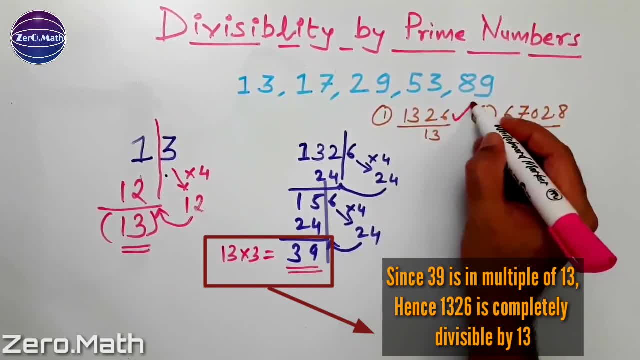 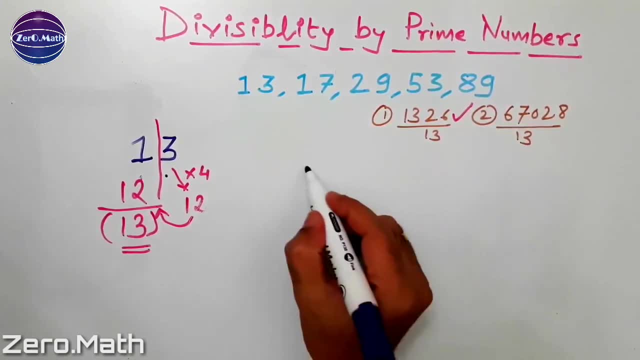 Because 13 into 3 is equal to 39. Again, 3 to 6 is completely divisible by 13. So let's take another example: 6, 7, 0, 2, 8. So let's apply the rule. 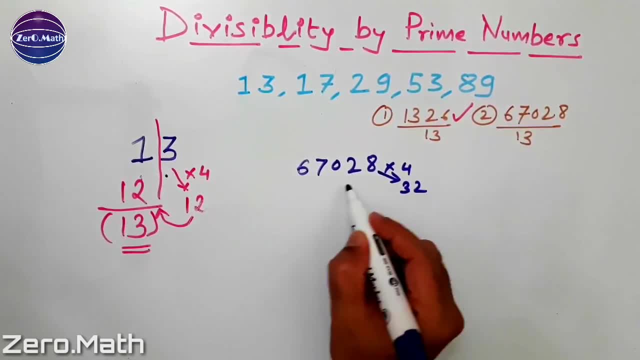 8 into 4 is 32.. So add this 32 over here, So 2 plus 2, 4, 3.. And 6, 7, 3, 4.. Again, apply the rule 4 into 4.. 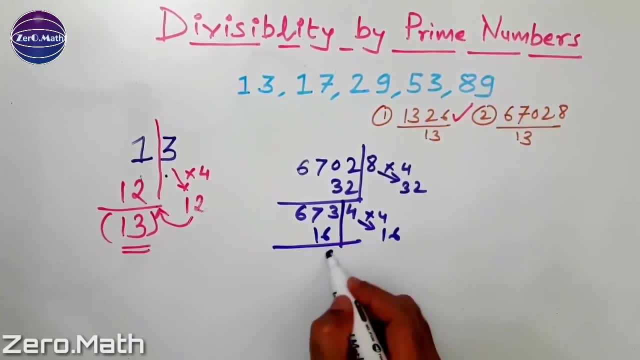 Is 16.. So add this 16 over here. 6 plus 3, 9.. 7 plus 1, 8. And 6.. 689.. Again, apply the rule 9 into 4: is 36.. 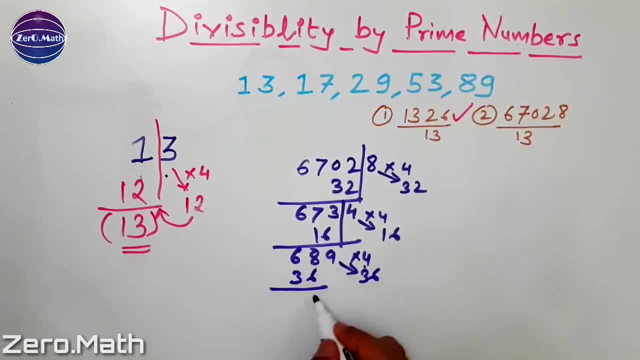 So let's add 36 over here: 6 and 8,, 14.. Carry 1,, 6,, 3, 9, 1, 10, 1, 0,, 4.. So apply the rule once again. 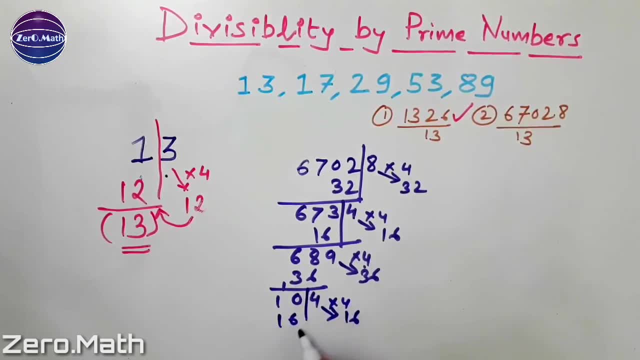 4 into 4 is 16.. So add this 16 over here. So 6 and 1 plus 1 is 2.. So you can see 26,. 13 into 2 is equal to 26.. Hence this number is also completely divisible by 13.. 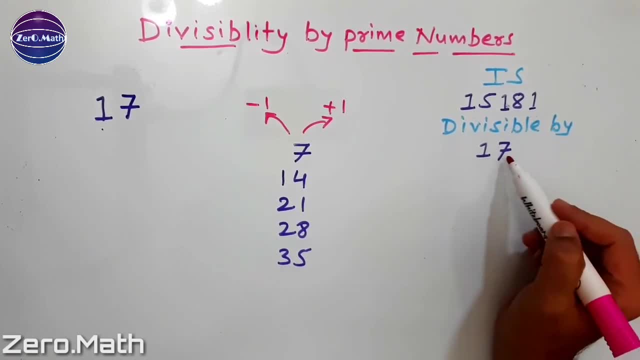 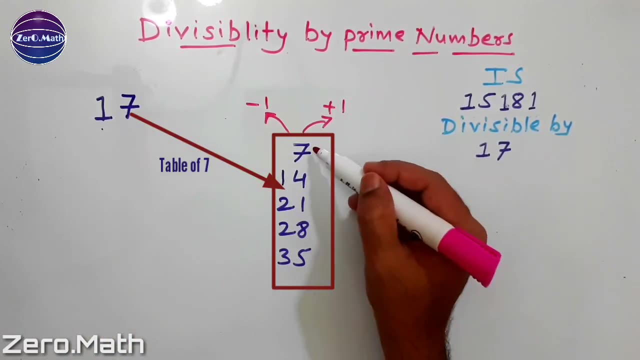 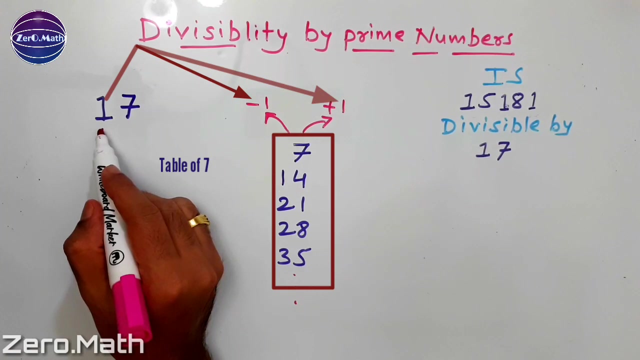 Let's figure out whether this number, 15181, is divisible by 17.. So let's first find out the divisibility rule of 17.. What I'm going to do, I'm going to write down the table of 7 here And I'm going to add or subtract this number, which is at the first place. 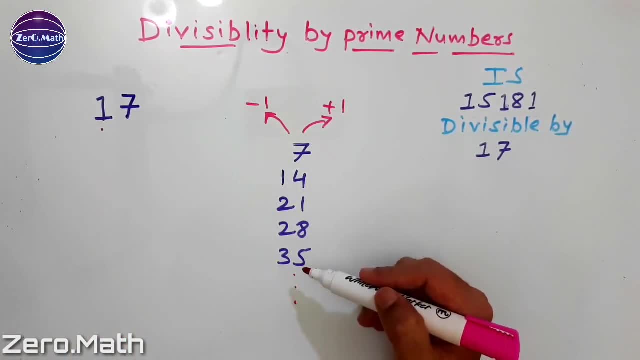 That is 1 from each of this number, so that I can get my answer as 17.. So basically, you can see: 14 plus 1 is 15, which is not equal to 17.. 21 minus 1 is 20, which is also not equal to 17.. 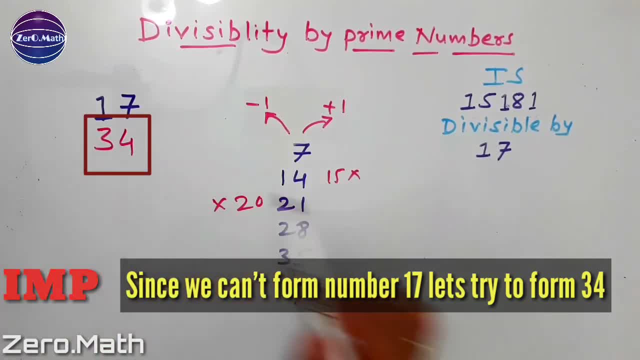 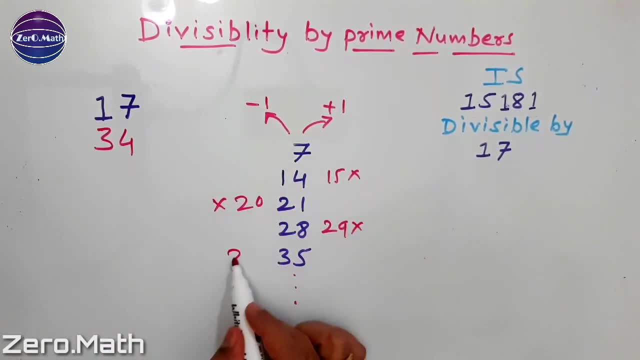 Since I'm not able to get 17,, let's try for 34, which is in multiple of 17.. So 28 plus 1 is 29, which is not equal to 34.. 35 minus 1 is 34.. So yes, here we get it. 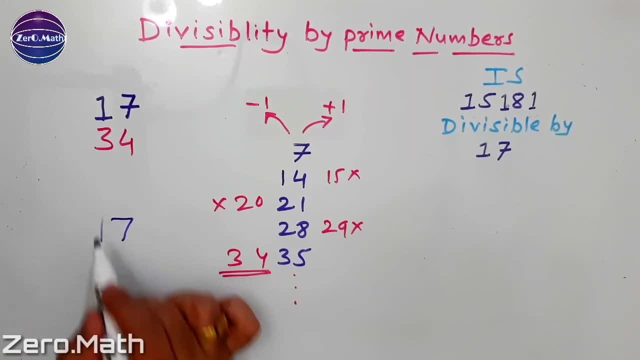 So basically the divisibility. So the divisibility rule of 17 will be: multiply this unit digit by 5, because 7 into 5 is 35. And subtract this from rest of the number so that we will get 34, which is in multiple of 17.. 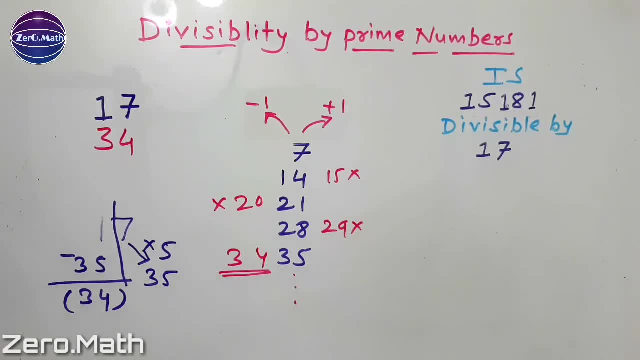 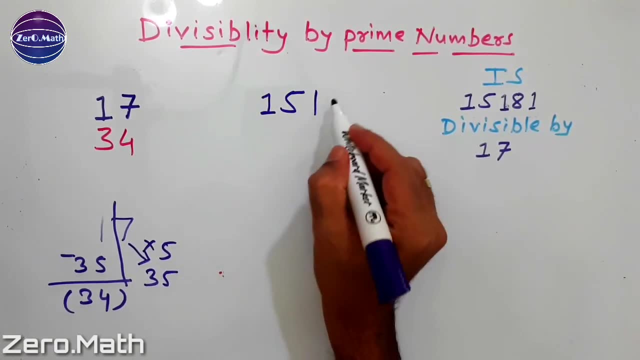 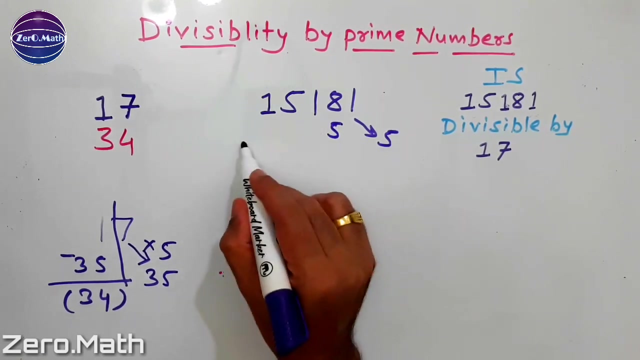 This is going to be the divisibility rule, So let's apply the rule now. Let's take this number, 15181.. Multiply the unit digit by 5.. So 5 into 1 is 5. And subtract it. So subtraction is most important, which you have to remember. 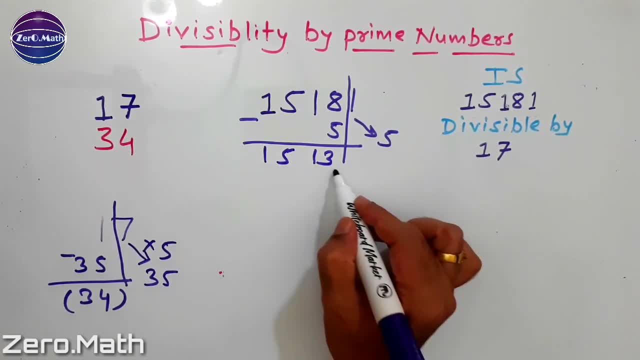 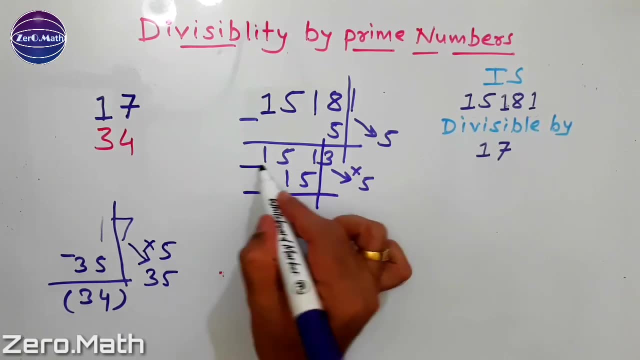 8 minus 5 is 3.. Rest of the number as it is. So again, 3 into 5 is 15.. So let's subtract this: 5, 6, 11.. So take 1, borrow: 5 minus 2 is 3.. 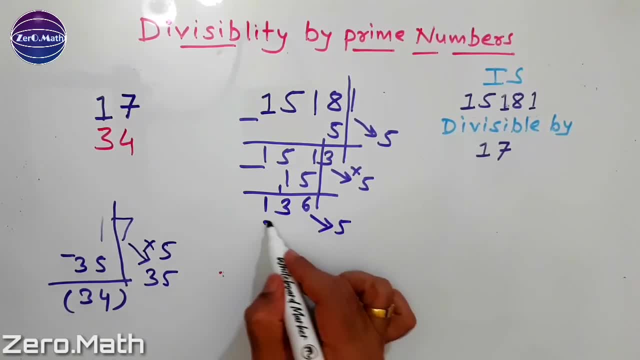 136.. Again, multiply this by 5, which is equal to 30.. So 30 minus 13 is 17.. So you can see: the result which we obtained is 17, which is in multiples of 17.. Hence, this number is completely divisible by 17.. 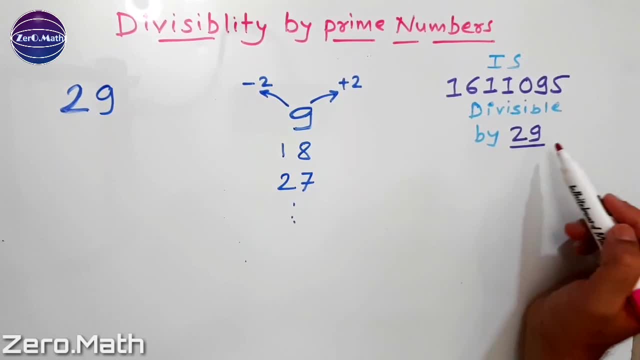 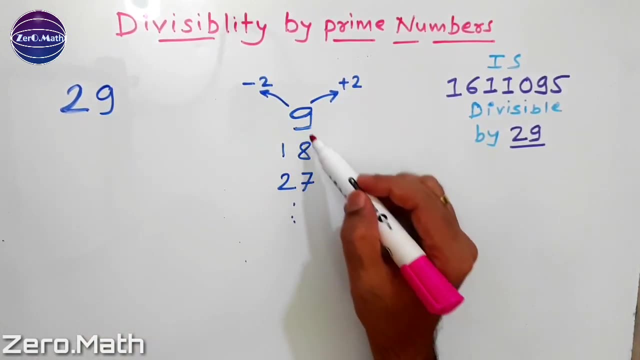 Let's try to figure out whether this big number is completely divisible by 29.. To do so, what I will do, I will take the unit digit of this 29, which is 9.. I will write down its table: 9,, 18,, 27, and so on. 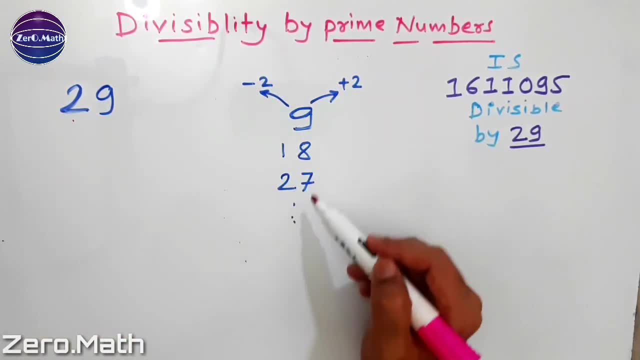 And 10 plus 18 is 2.. I will add and subtract from each of the number and try to figure out whether I can obtain this number 29.. So basically, you can see, 27 plus 2 is equal to 29.. So that's going to be my divisibility rule. 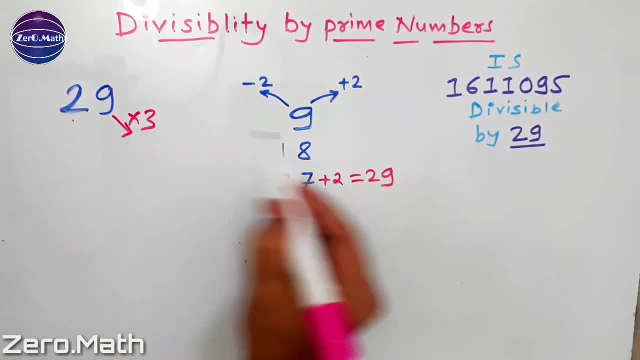 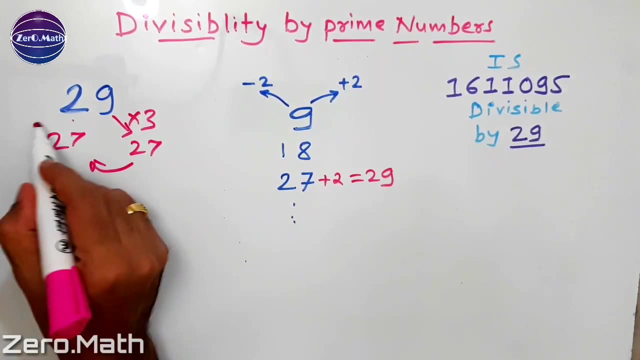 So simply what I will do: I will just multiply this 9 into 3. Because this 27 is 3 times 9, which is equal to 27. And add this 27. To rest of the number And, after doing this, if the result which I am getting is in multiple of 29.. 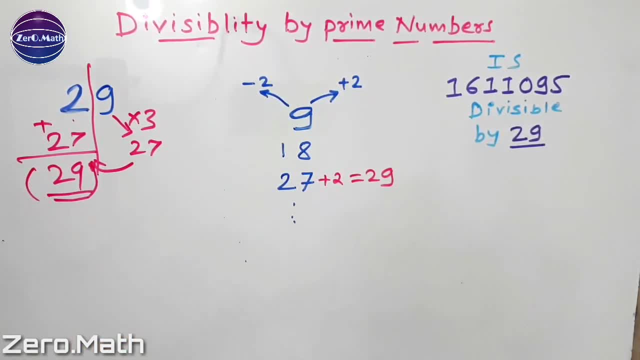 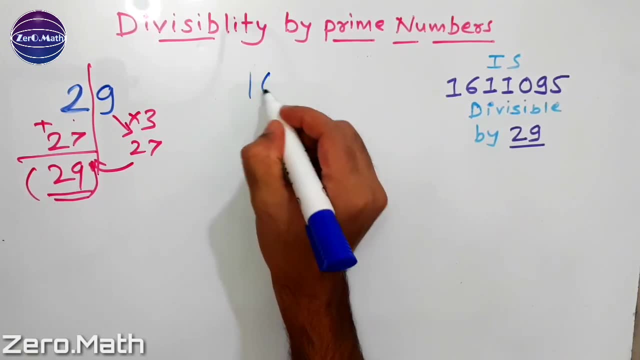 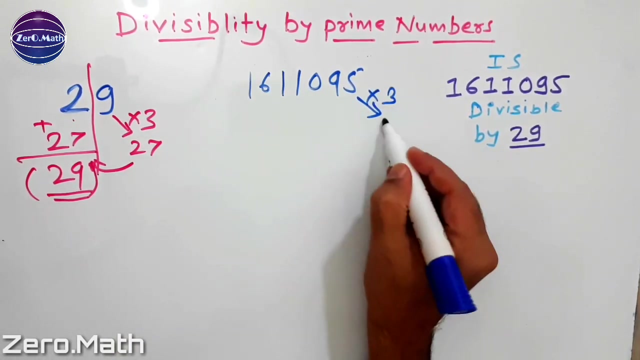 Then, yes, my number is going to be divisible by 29.. So let's solve this example. So let's take this: 1611095.. Apply the rule So unit digit into 3, 5 into 3 is 15.. 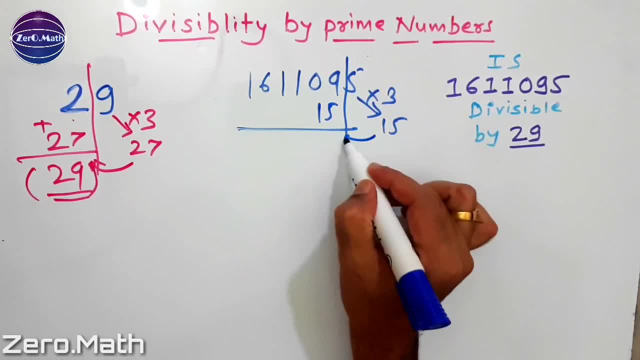 So I will take this 15 over here And 9 plus 5, 14,, 1,, 1, 2, 1, 1, 6, 1.. Again, multiply the unit digit by 3, 6,, 4 into 3, 12.. 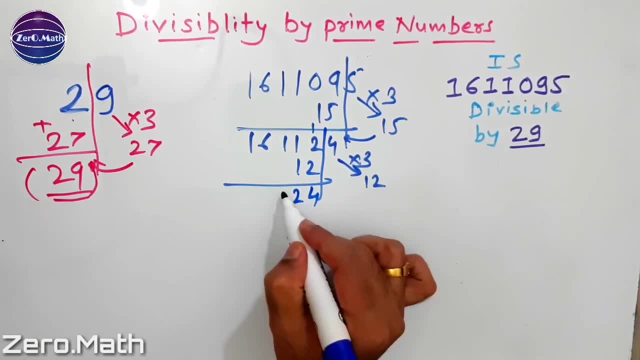 Add this 12 here: 2, 2,, 4,, 1, 1, 2,, 1,, 6, 1.. Again, multiply it by 3.. So 4 into 3 is 12.. So which is equal to 2, 2,, 4,, 1,, 1,, 2,, 6, 1.. 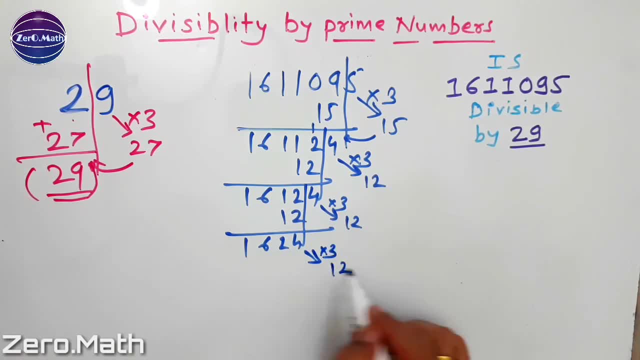 Again, multiply this unit digit into 3.. 4 into 3 is 12.. Add it here, So 2, 2, 4, 6, 1, 7 and 1, 74.. Again, 4 into 3 is 12.. 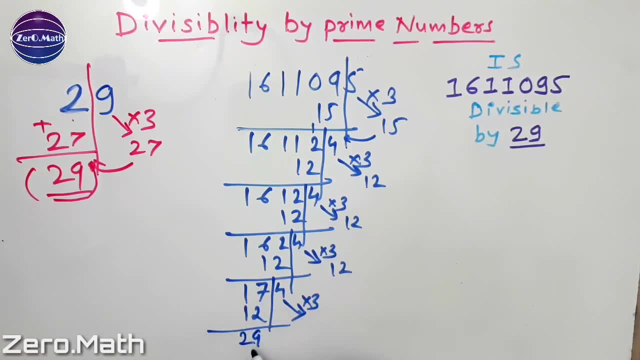 So 7 plus 2, 9.. 1 plus 1, 2.. So what result we have got is 29.. Since the result is in multiple of 29.. We can say this number is completely divisible by 29.. 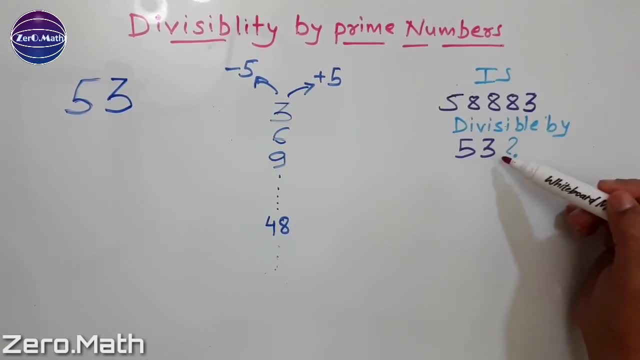 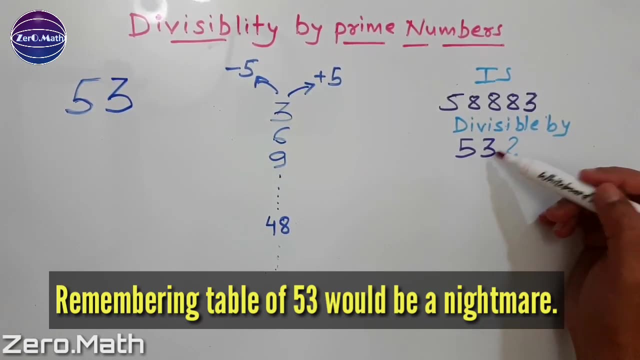 Friends, let's try. Let's try to figure out whether this number is divisible by 53.. So it's very difficult for you or for anybody to remember the table of 53. So let's find out the divisibility rule of 53.. 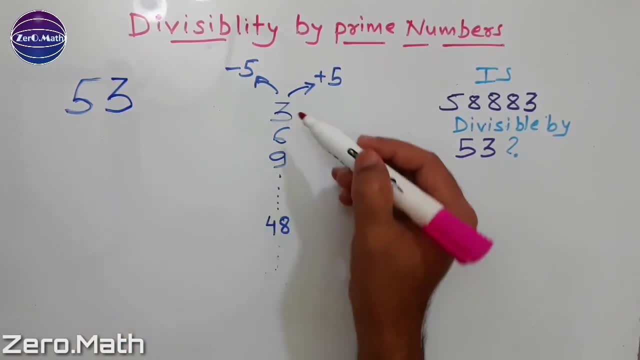 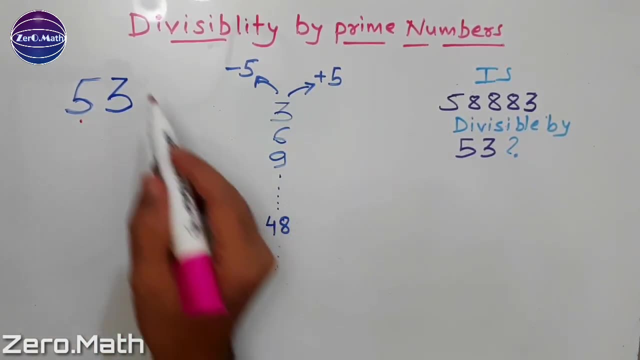 I have taken this number which is at the unit place, that is, 3.. And I have noted down its table And I am going to add the number which is at 10th place, that is, 5, to each of the number, So that I can form this figure: 53, or the multiple of 53. 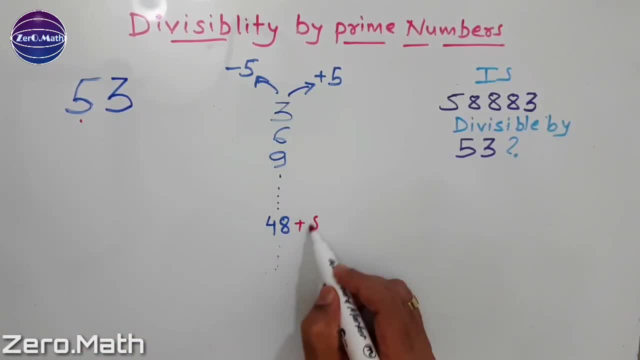 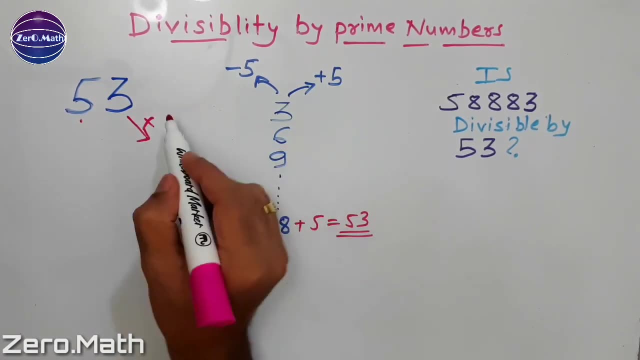 So basically, you can See 48. if I add this 5 to 48, I am going to get 53.. So the divisibility rule will be 3 into 16.. Because 48 is 16 times 3, which is equal to 48.. 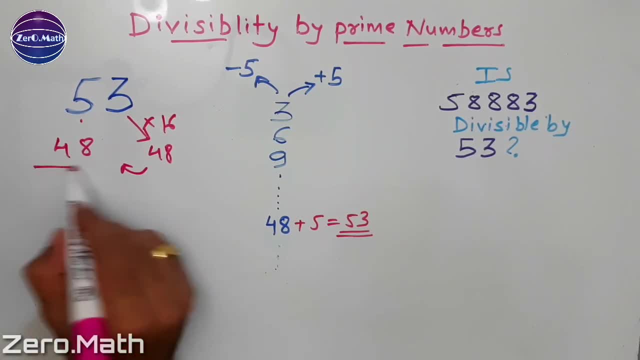 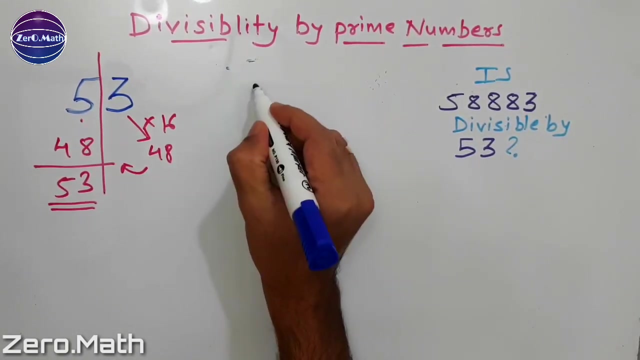 And add this 48 to the rest of the number, so that you can get 53., Which is completely divisible by 53. So that's going to be our divisibility rule. Let's test it. So: 5,, 8,, 3.. 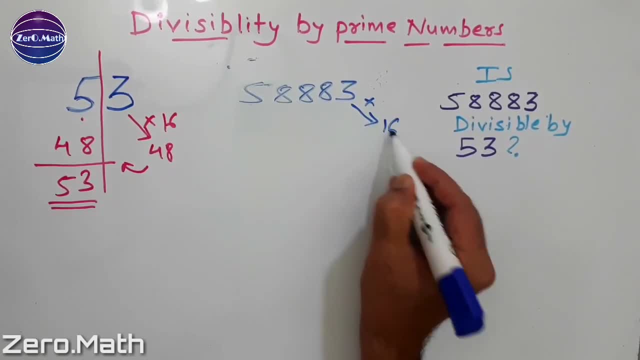 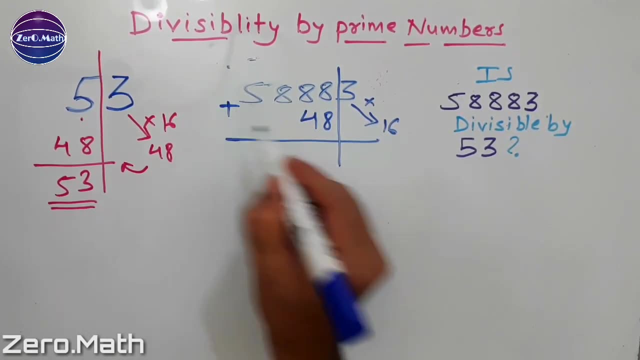 Let's multiply this unit digit into 16.. So 16 into 3 is 48.. So let's add this 48 here. 8, 8, 16. Carry 1.. 8,, 4,, 12 and 1, 13.. 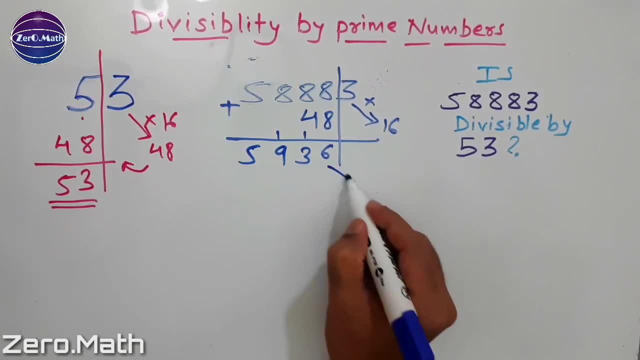 Carry, 1.. 8 plus 1, 9.. 5,, 9,, 3, 6.. Again, multiply this 6 by 16. So 16 into 6 is 96. So 6,, 3,, 9.. 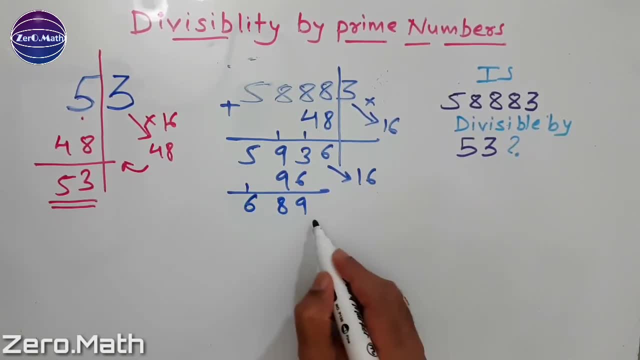 9, 9, 18. 8. Carry 1. 5 plus 1, 6. Multiply this 9 by 16. So 16 into 9 is 144.. So 8, 4, 12.. 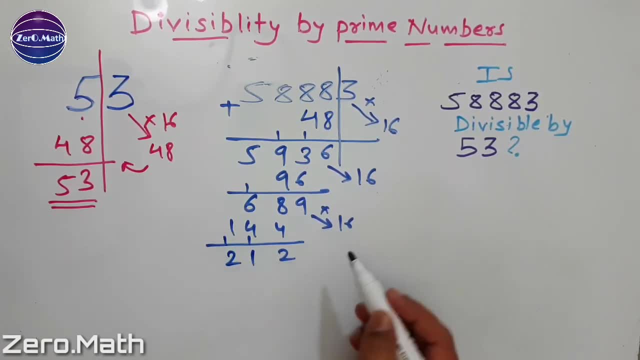 6,, 4,, 10. And 1, 11. Carry 1. 1 plus 1, 2.. So 2, 1, 2.. Let's apply the rule again. Multiply this 2 by 16.. 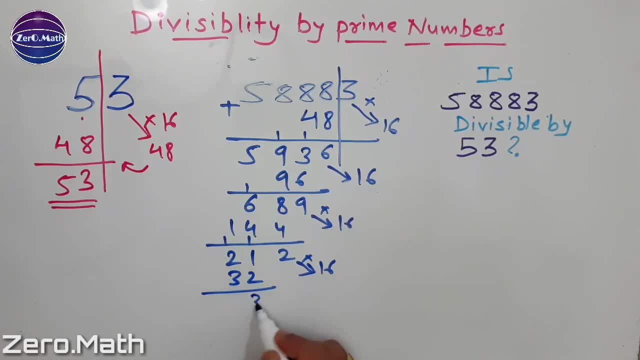 2 into 16 is 32.. So what I got? 2 plus 1, 3.. 3 plus 2, 5. Which is equal to 53.. Which is in multiple of 53. So that we can say this number is completely divisible by 53.. 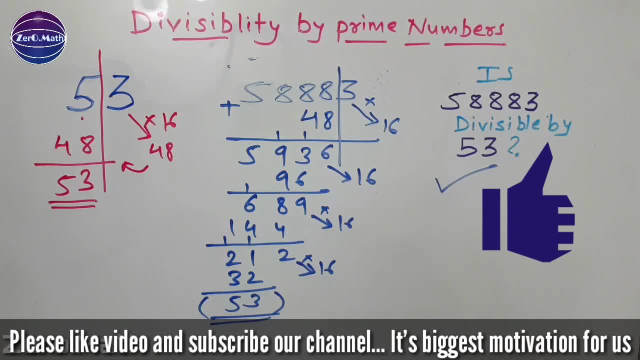 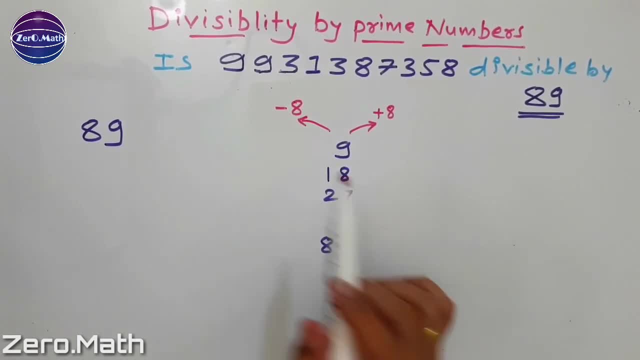 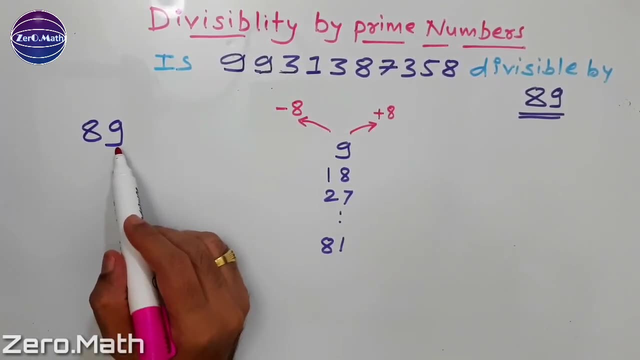 I hope you got this concept And you can see how easy we have made it using this divisibility rule. So, friends, let's figure out whether this big number is completely divisible by 89.. First, find out the divisibility rule of 89.. 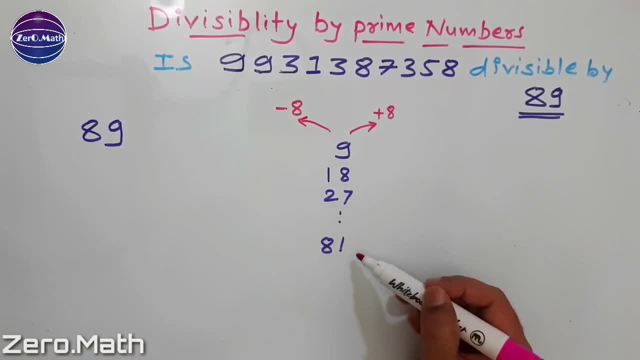 So, to do so what I will do, I will write down the table of 9, which is at a unique place, And I will add- and I will try to figure out whether I can get number as 89.. So basically, you can see, 81 plus 8 is equal to 89.. 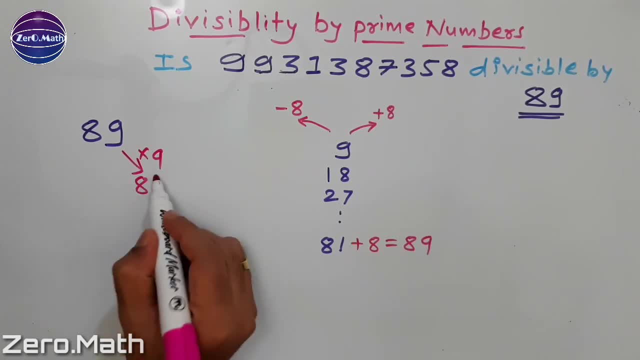 So, which means 9,. when multiplied 9 times, I will get 81. And I will add this 81 here so that I can get 89,, which is in multiple of 89. Hence, this is going to be my divisibility rule. 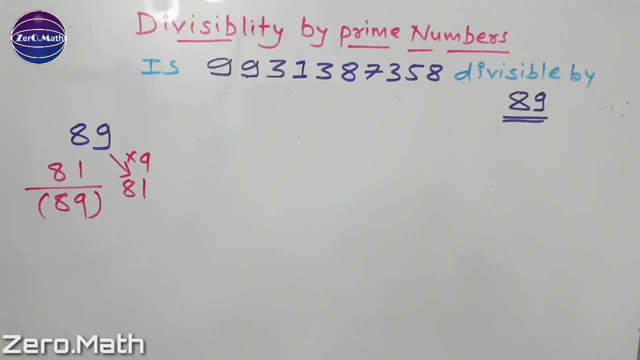 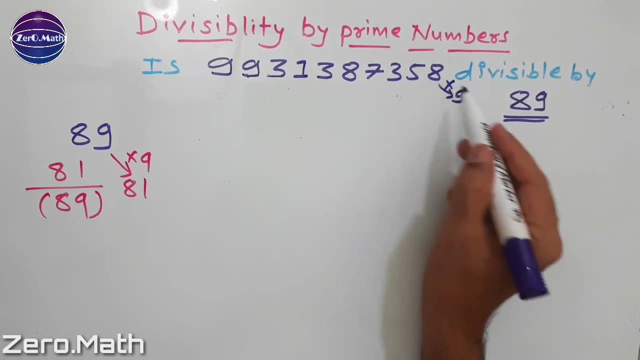 So let us test it. Let's multiply this unit digit number by 9.. So we will get 9 into 8 is 72.. Let's add it: 5 plus 2, 7.. 7 plus 3, 10.. 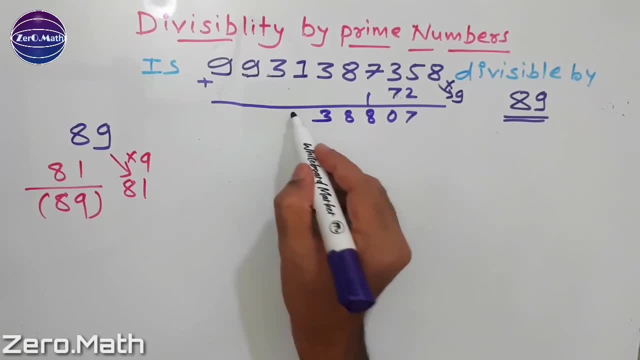 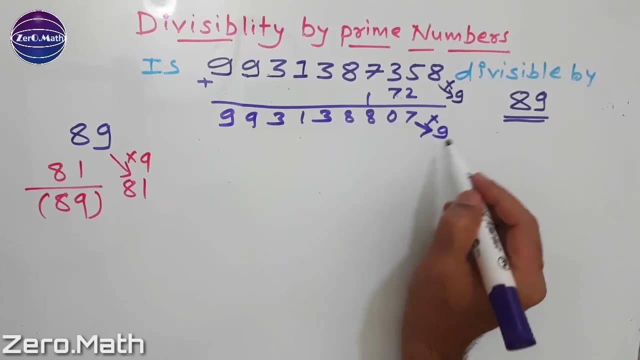 Carry 1, 7, 1, 8.. Rest of the number as it is. Again, multiply this 7 by 9 and add it to the rest of the number, So 7,, 9,, 6,, 8,, 3.. 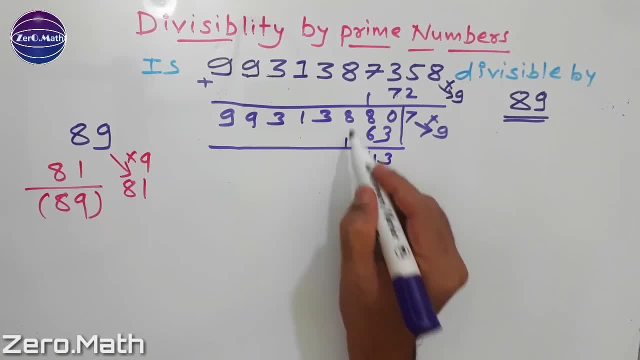 Let's sum it up: 3, 8,, 6,, 14.. Carry 1, 8,, 1,, 9.. 3, 1,, 3,, 9,, 9.. Let's multiply this 3 by 9.. 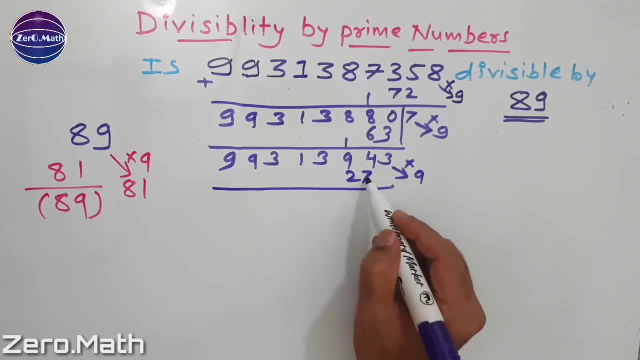 So 9 into 3 is 27.. Add it to the rest of the number 7,, 4,, 11.. Carry 1,, 9,, 2,, 11 and 1, 12. Carry 1,, 3,, 1, 4,, 1,, 3,, 9,, 9.. 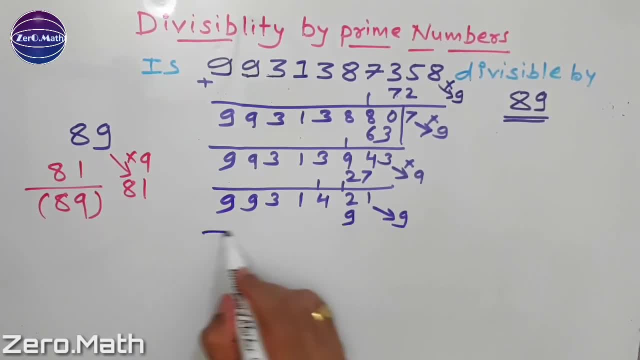 Again, multiply this, Again, multiply this, Multiply it by 9.. So it will become 9 plus 2,, 11.. Carry 1, 4 plus 1, 5.. 1,, 3,, 9,, 9.. 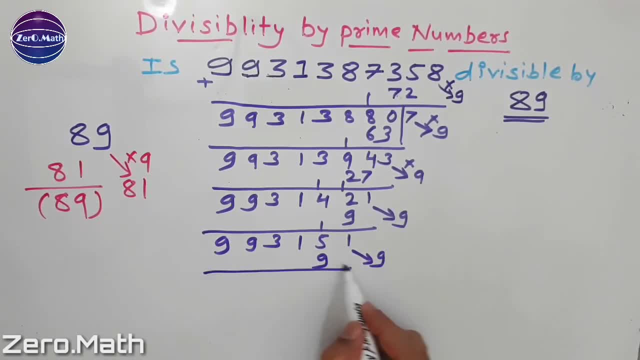 Again, multiply it by 9.. So 9,, 5,, 14. Carry: 1,, 1,, 1,, 2.. 3,, 9,, 9. Again, multiply it by 9.. 9 into 4 is 36.. 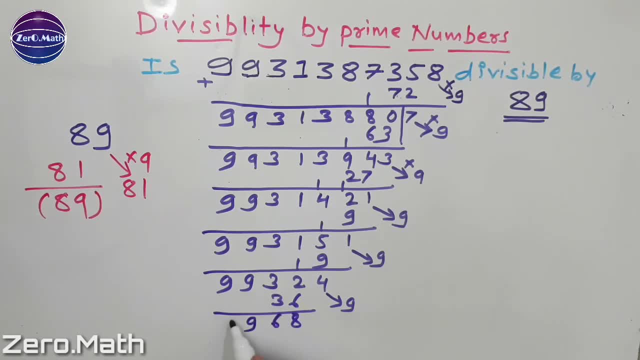 6 to 8.. 3 plus 3, 6.. 9,, 9,, 6, 8.. 9,, 9,, 6, 8.. Take this number here: 9, 6, 8.. 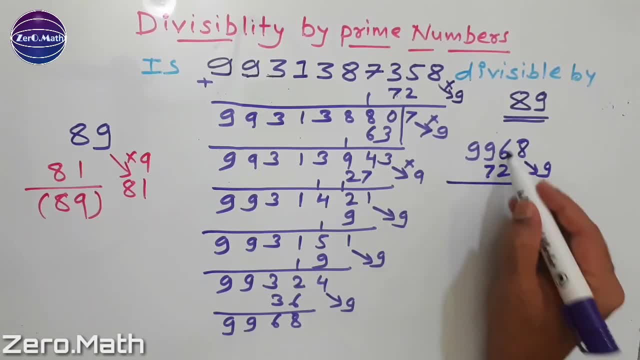 So 8 into 9 is 72.. 6 to 8.. 9 plus 7 is 16.. Carry 1, 9 plus 1, 10.. 1, 0, 6, 8.. Again, 8 into 9 is 72..